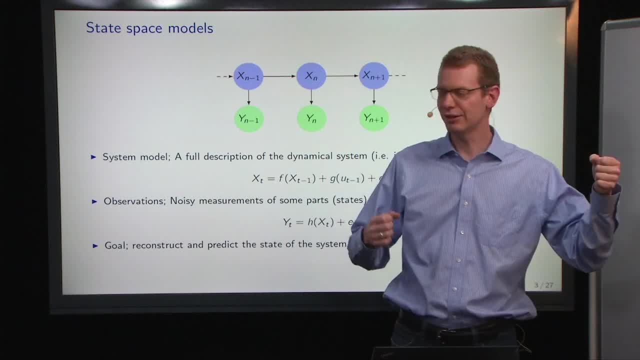 temperature of a house. You have a thermometer someplace here, maybe there, but you don't have the temperature in your house. You don't have the temperature in your house. So what you would do is you would have a thermometer somewhere here, maybe there, but you don't. 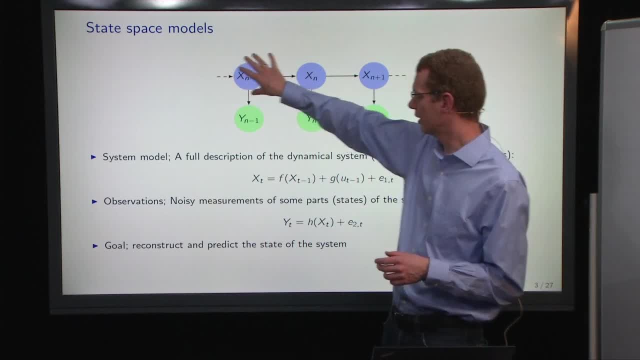 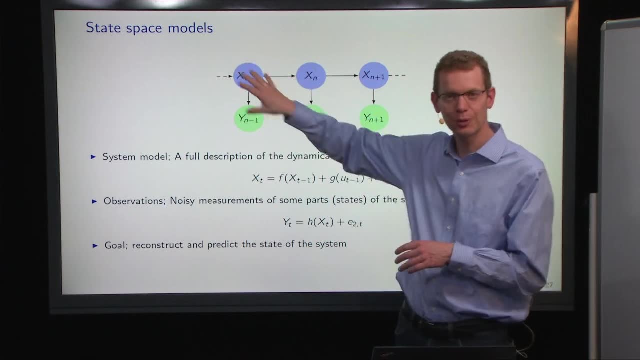 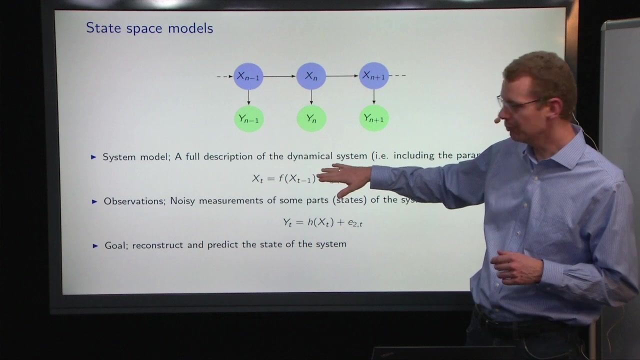 have it everywhere. So you have an underlying model, that is the house, and then you have some observations somehow, And the question is then how to make a model for the house. but that's a different story. But we have, in general, a full description of the dynamical. 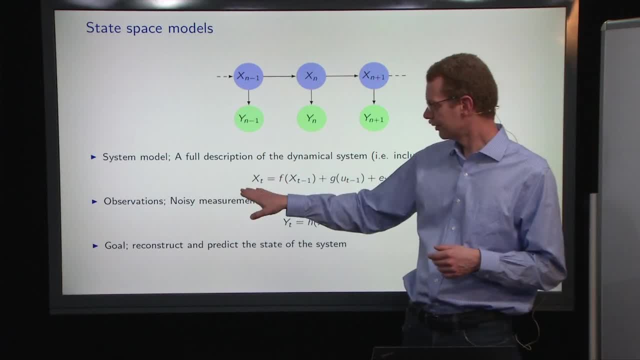 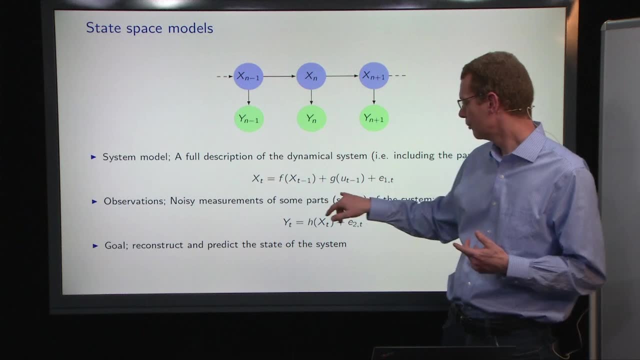 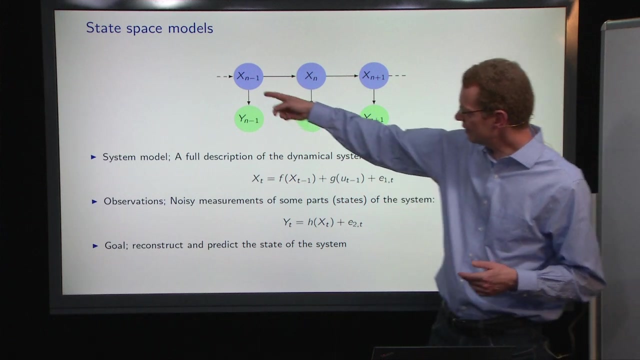 system, say the heat dynamics of a house, where at x, t the state of time t depends on the function of the previous state, plus the function of an input, plus potentially some noise. Now the observation equation indicated by this arrow here is then a nonlinear potentially. 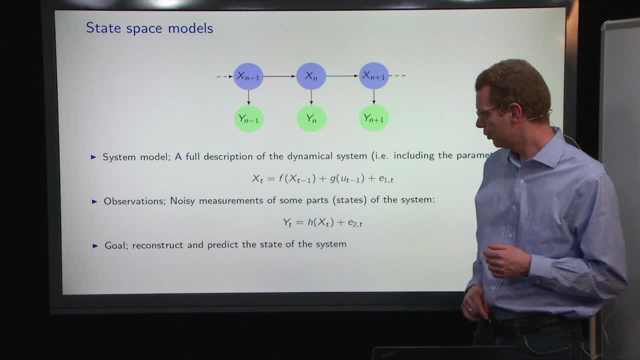 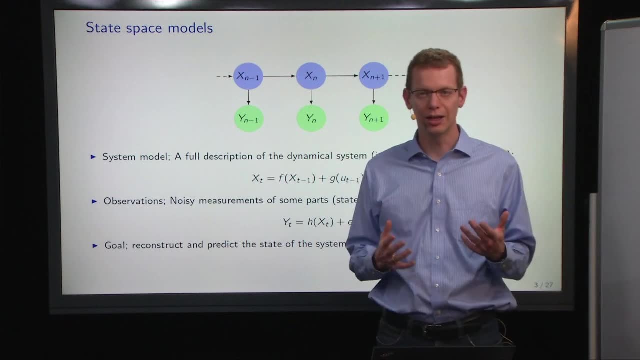 nonlinear function of the input given, as the output y, t plus some observation noise, And the goal here is to reconstruct, as in update, our estimator of where we are given new observations, So whenever we have. 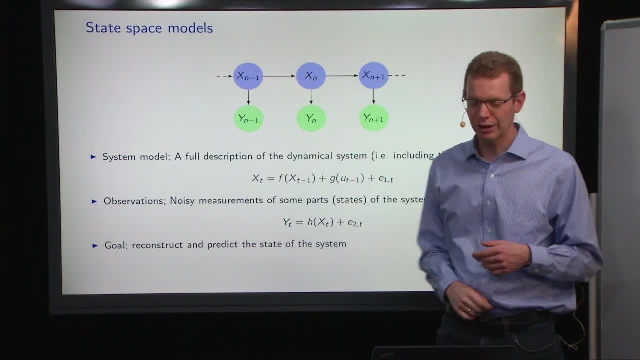 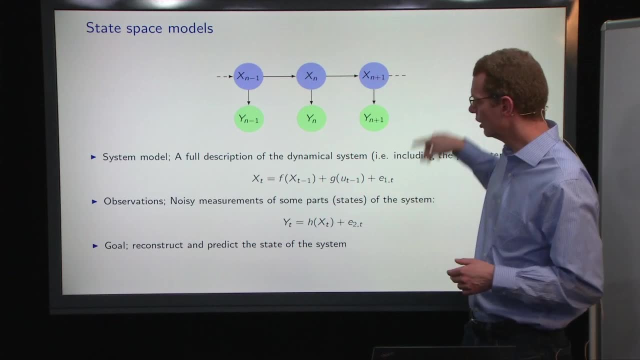 serve y. in say we want to say, well then, what more do we then know about the state of the system at that time? But we also want to make predictions of the future. That's all that we want Now. since this is linear time series calls, we will have these as only. 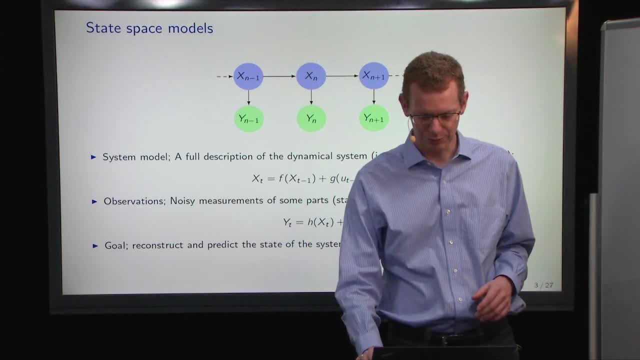 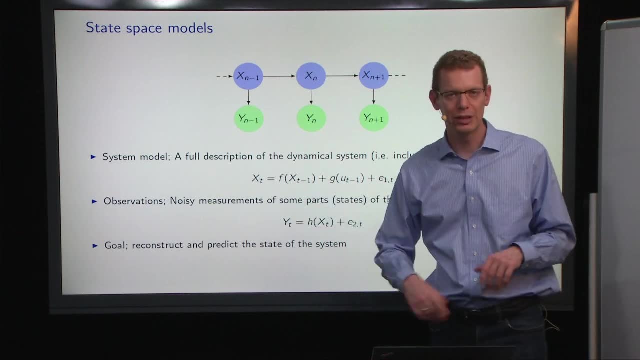 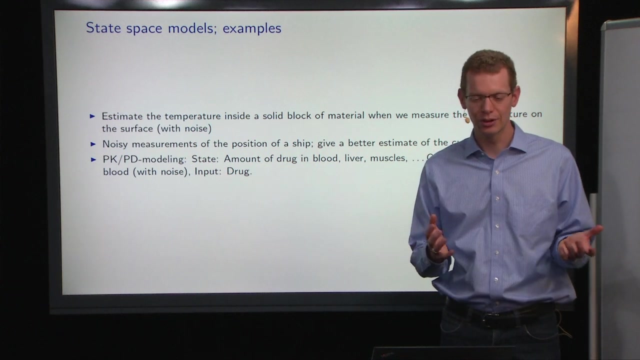 linear functions. but this is a general state space representation. The big difference to what we've done so far is that it only depends on the previous state, which means it also mark of property. Just a couple of examples: I mentioned the temperature of a house. it could be a temperature. 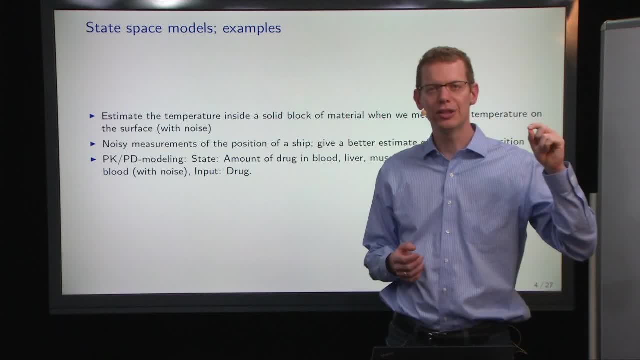 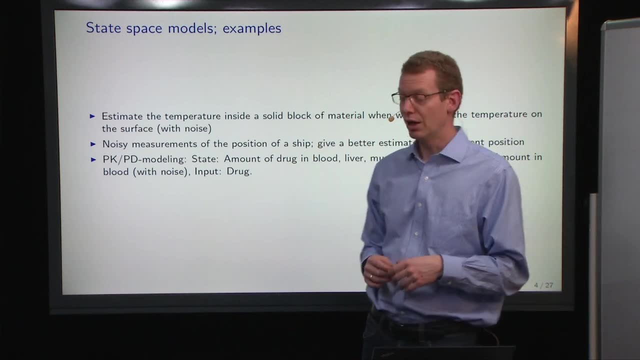 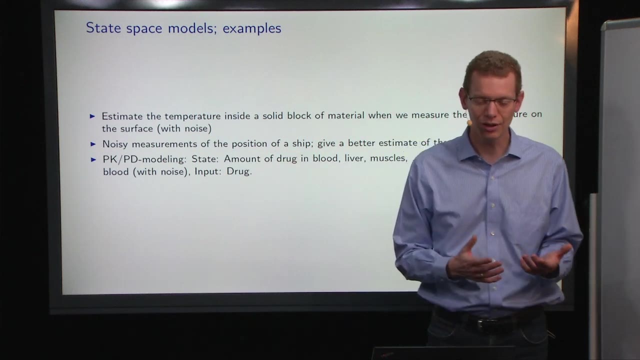 of anything. but what is typical there is that you measure the temperature somewhere and you think of it representing the entire thingy. Now, another case would be, well say, the precision observations. they could be noisy. Now with GPS, they're not as noisy, but you should also keep in mind that GPS fails. so 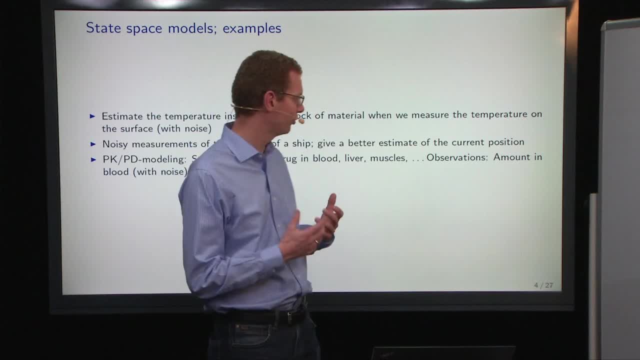 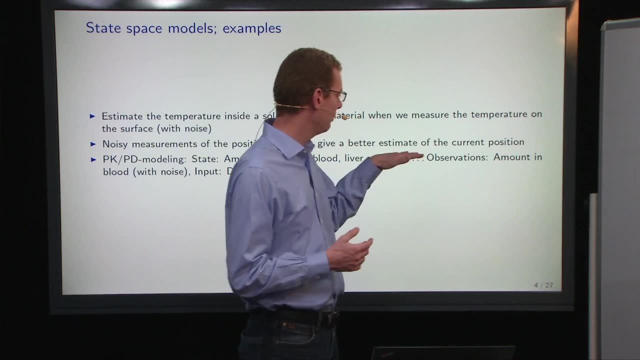 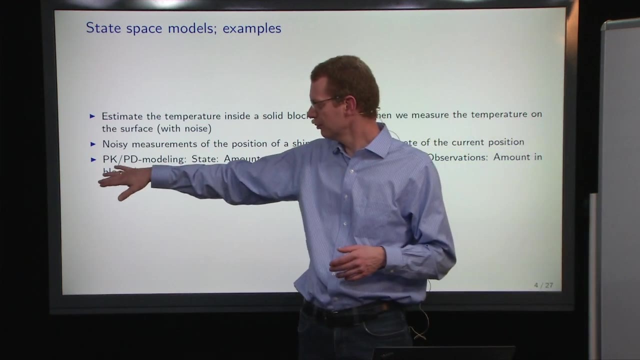 whenever we have other systems, you need to have an understanding of the uncertainties. So the idea is: given many observations that have some noise, we may be able to combine that into a better estimate of the precision In biological system. what is medical research? one very important class of models are the 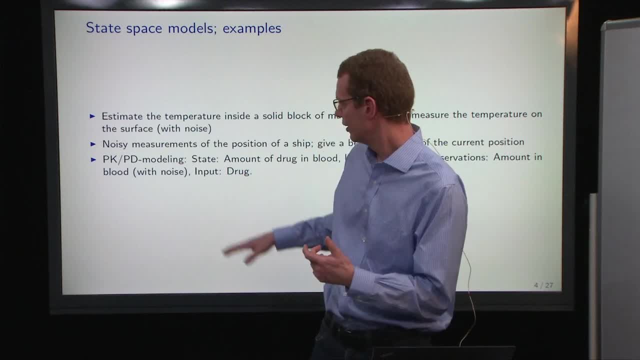 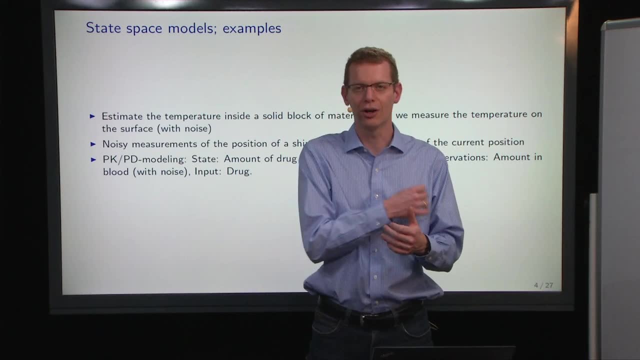 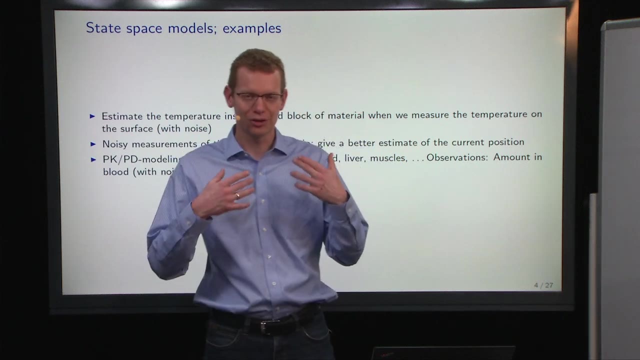 so-called pharmacokinetics and pharmacodynamic models, where the kinetics are how is a drug diluted in the body, And the dynamics are pharmacodynamics- how is the drug then active where it is Now? I hope that you can follow me in thinking that when you want to describe that, if you. 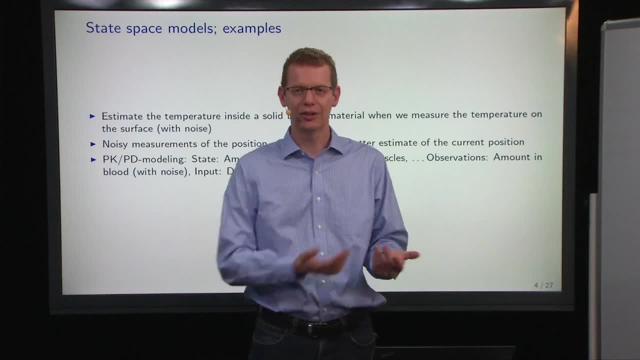 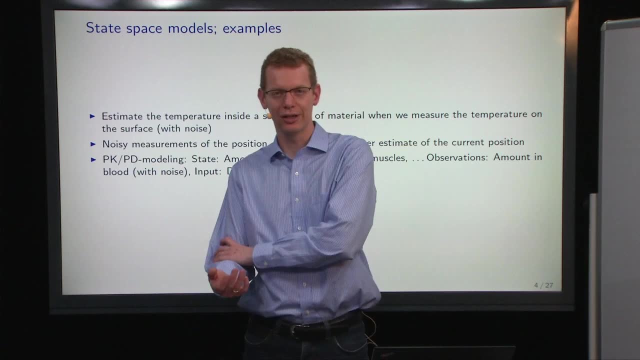 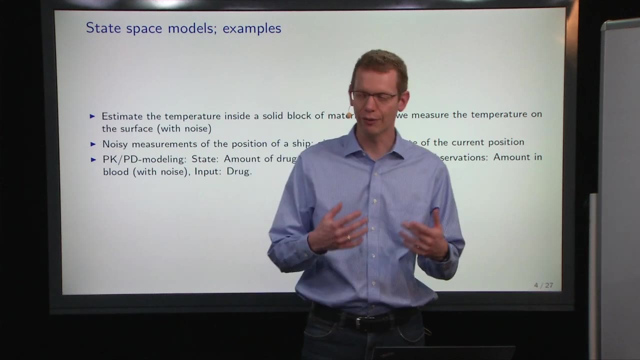 inject something somewhere, it's not everywhere immediately. it takes some time to get through the system. On the other hand, when you make observations of the concentration profile, you may do that in the alarm, but you're not doing it everywhere, So you're measuring somewhere with some noise and delays and other things that you have. 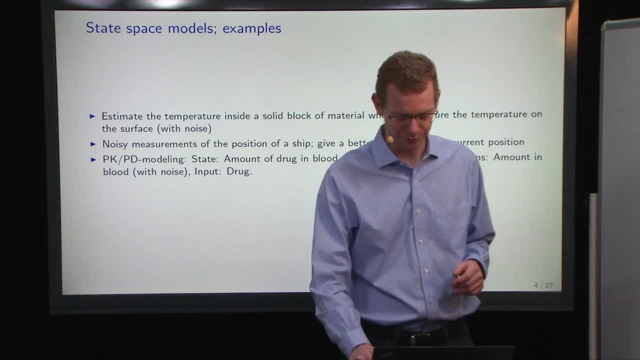 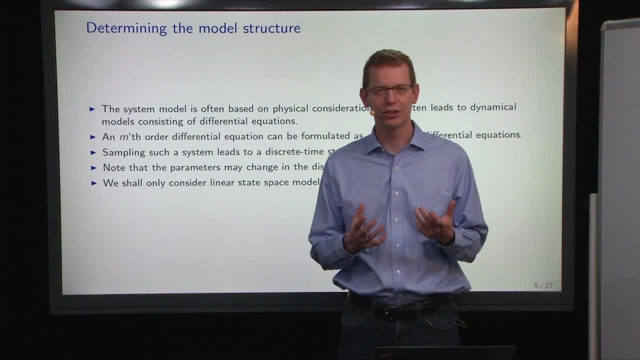 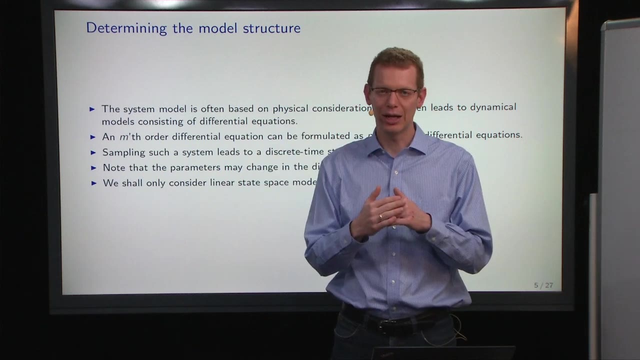 to include, And that's what you want to do in your model when you're doing the modeling. So what we have to do here is that we have to consider the physics of the system that we're looking at. So what are the governing states that we have to control, say, for the blood or for the body? 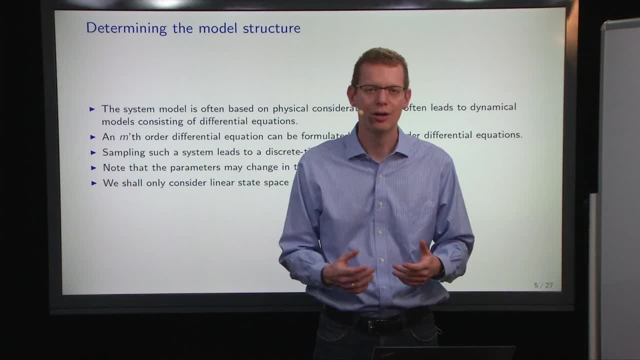 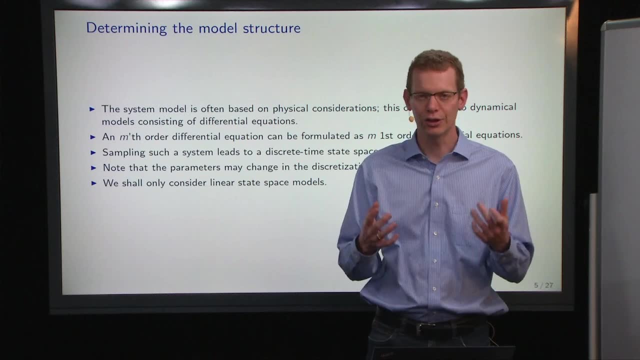 We have the bloodstream and then we have the tissue, and maybe we need more for the local about where the injection is and other things. Again, it depends on understanding that. Okay, So the physical or physiological system that we're modeling, this is what we call going. 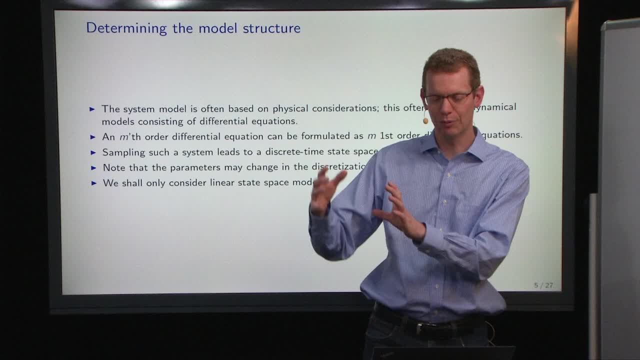 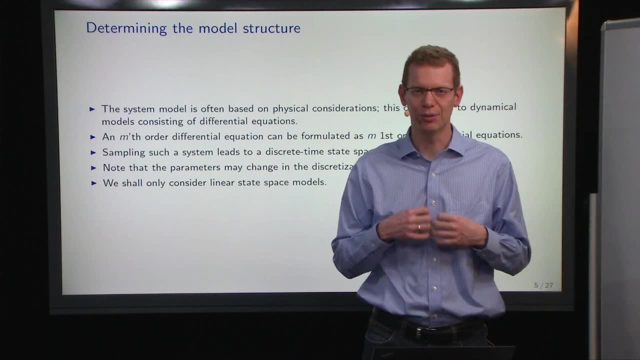 towards having a white box model where we try to describe as much of the model as we know. But on the other hand, as I said before, there are other things where we say we don't want to model every single vessel, blood vessel in the body. 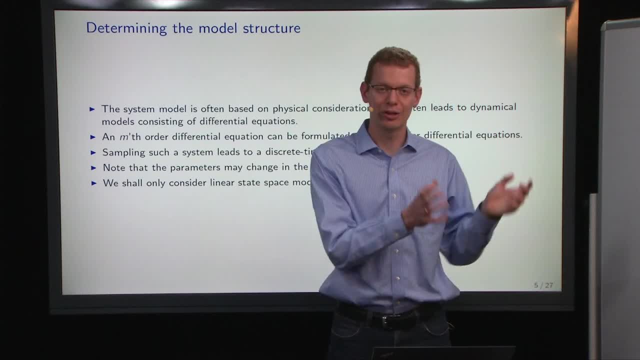 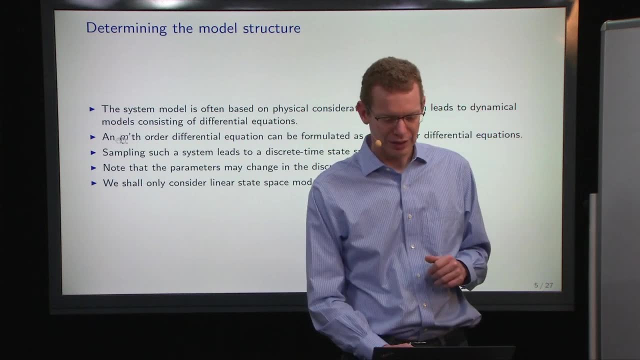 So we also want to use- you can say some of the noise can be used to kind of reflect the things that are not covered by the model. Okay, Okay, Okay. So the first thing is that you can take any mth order differential equation and then you 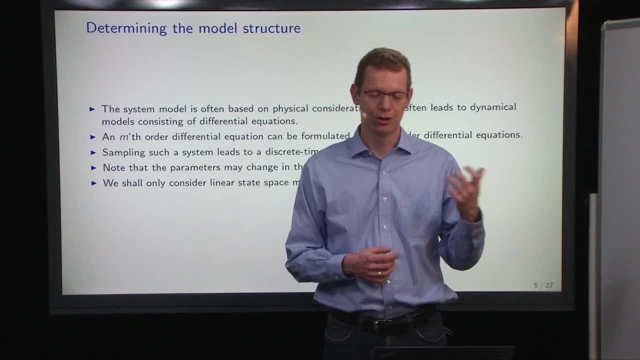 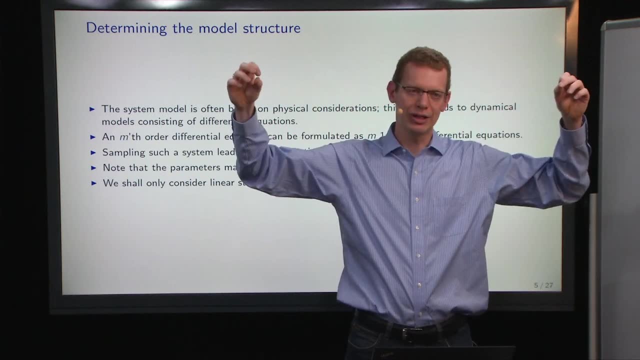 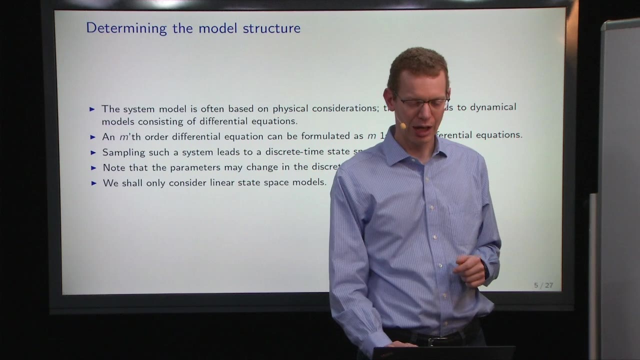 can formulate that as m first order differential equations. The typical thing is that you take a acceleration model for the second order, derivative acceleration of something and then you write that as two coupled first order differential equations. And the other thing in that regard is: whenever you do observe a system, it's almost always 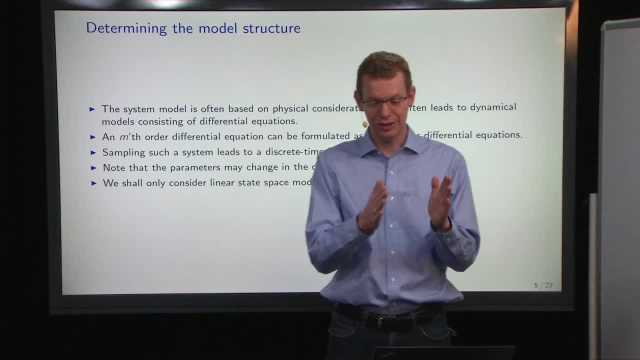 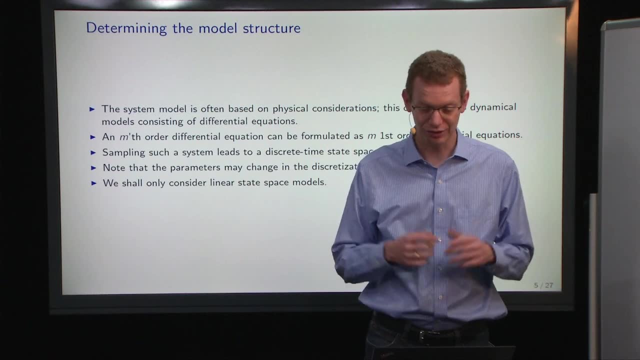 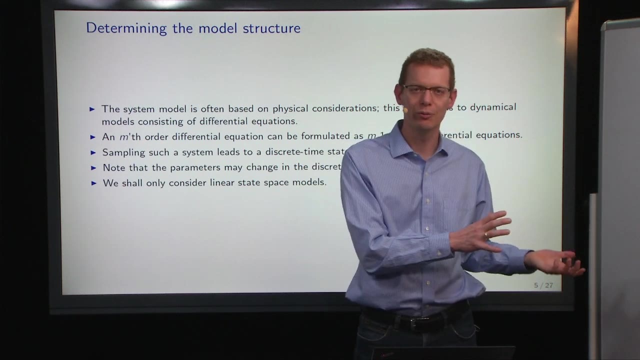 in discrete time. Okay, So if it's equidistant, then we're in the scope of this, but we can also handle non-equidistant distance samplings. But you should also keep in mind that when you do this change from continuous time to. 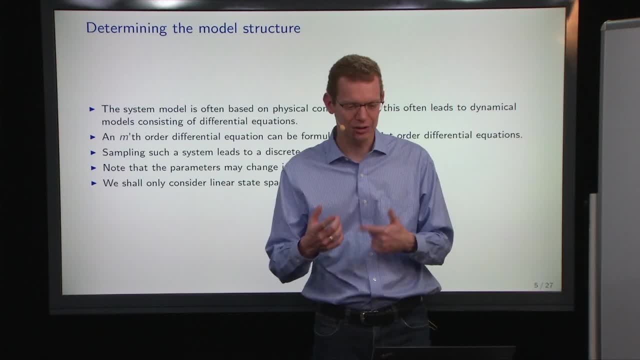 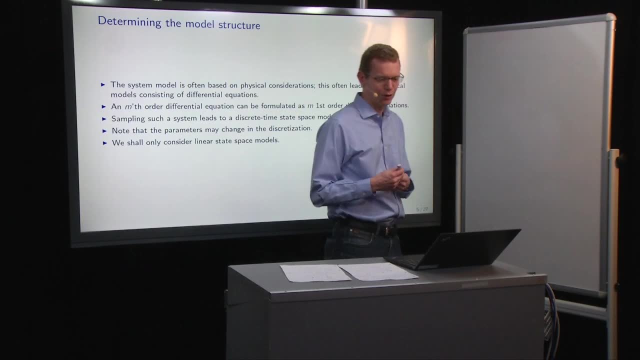 discrete time. you may also change the prioritization in the model. We'll get back to that. But let's first just see how that happens for a simple differential equation. If we write dx, dt equals a times x, then I hope that you all know what the solution 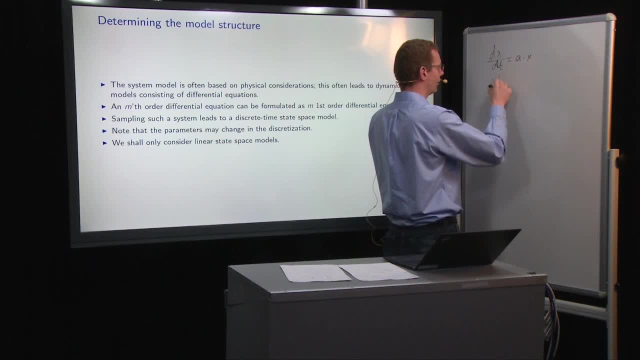 is to this equation, namely that x at time t equals sum x zero. let's call it that times the exponential of a times t. Now, if you want to do this in discrete time, what we're looking at, we could say that if 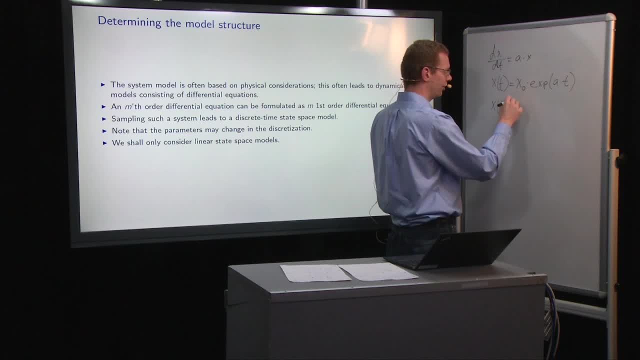 we look at x at time t plus delta t and we just plug that in up there. then we have x naught times exponential of a times t plus delta t. Now if we look at this, we can take the sum in here and split it out. so we have that. 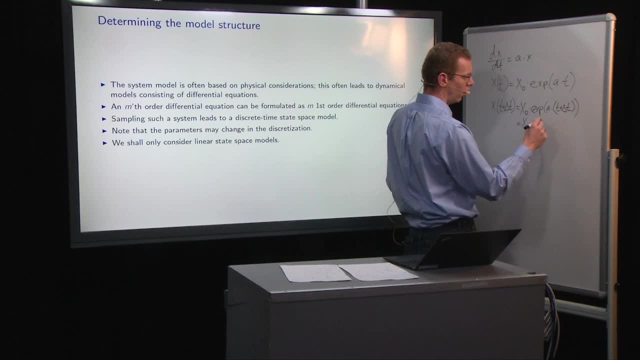 as x naught, And what we see here is that times equal to the exponential of a times t, and we multiply that by the exponential of a times delta t. Now, what we do see here is that we will identify the first bit here. that is exactly what we. 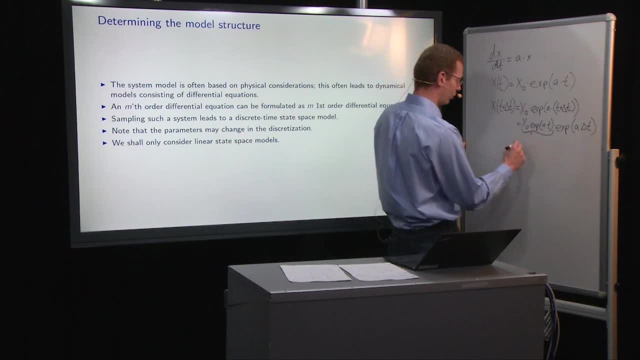 have up here as xt, So at xt plus delta t, what we have is what we've already got from that first step, which is impatient: x of t. and then we have it: times the exponential of a, times the sampling period, delta t. So if you want to write this in a discrete time manner, a similar.